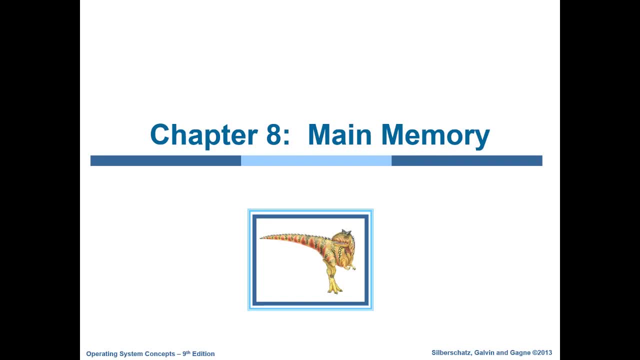 so chapter 8 is about main memory. okay, and we know about the importance of main memory. we know that if any computer system does not have main memory, then you cannot run programs, because if you are programmed in the hard disk and you want to run it in the CPU, then this program must be. 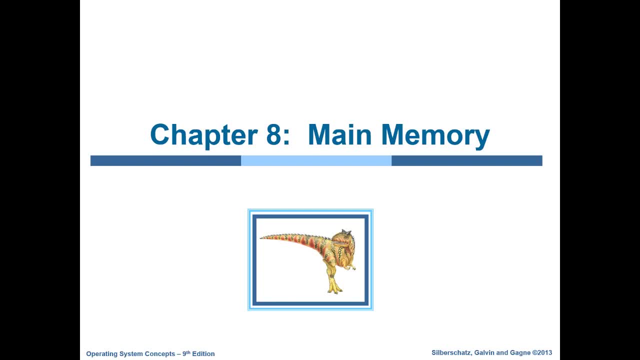 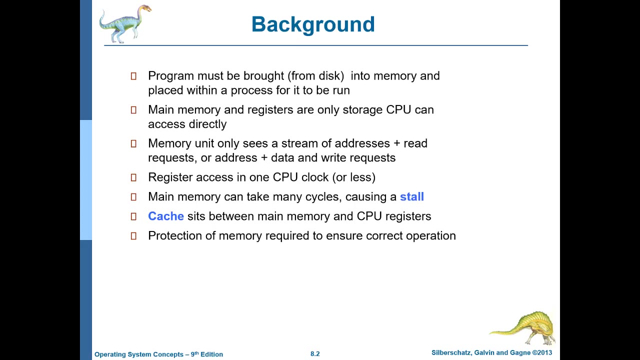 first brought into the main memory to make a process and then the CPU executes the instructions of the process from the main memory. this is the importance of main memory. now for a CPU, it can only access registers and main memory. now for main memory, it has only the information about addresses. main memory only knows that it has a set of 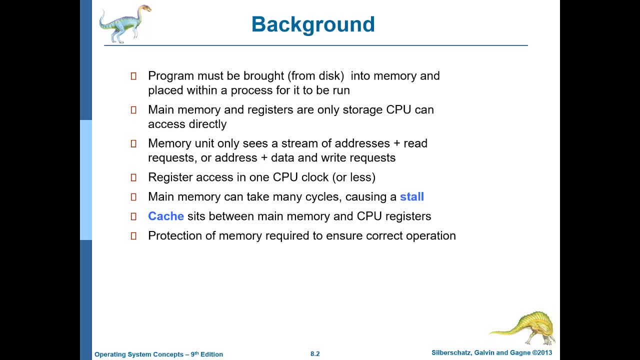 addresses: okay, that starts from zero until the size of the memory. okay, and whenever CPU requests to read something from main memory, it will give the read request and the addresses from which to read. or if the CPU wants to write something into the memory, okay, saving some data into main memory because the user makes some changes, then the CPU will set. 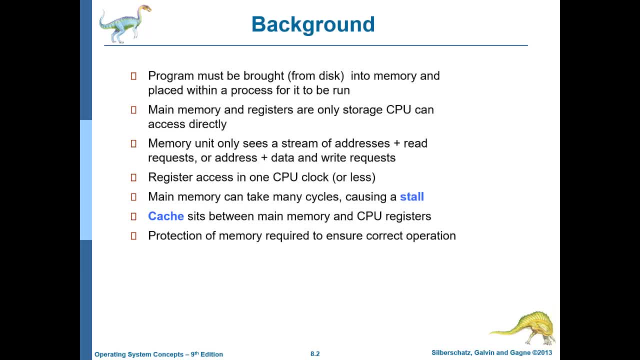 the addresses. it will send those addresses to the memory unit in which to write and it will also send the data to be written into those addresses. now one issue is that if the CPU accesses data from the register, then it can be done in one CPU clock, but if the data is to be accessed in main memory, then 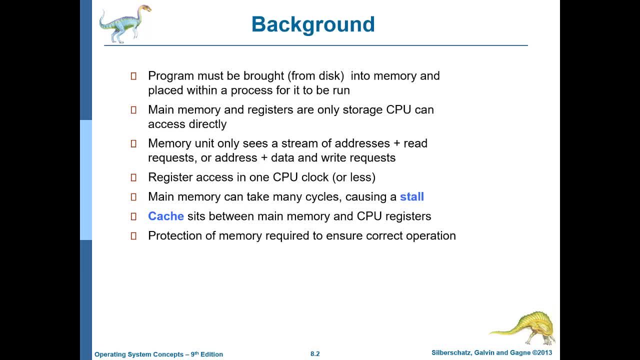 it can take many cycles and this time taken for many cycle. this is actually known as a term which is called stall- memory stall- to reduce the memory stall. what we do normally is that if we have CPU, okay, let me draw this for you. if we have CPU, okay, this is my CPU and this CPU is on a chip. 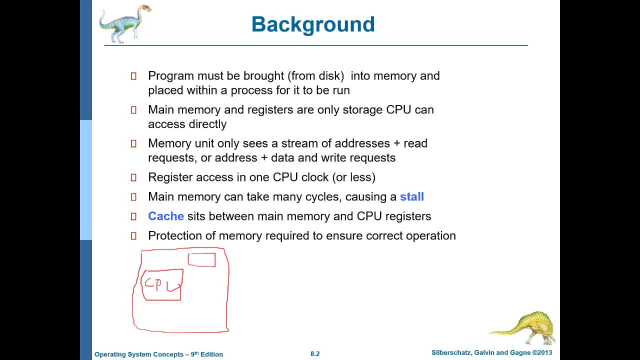 okay, and there are registers in the same shape. okay, these are different registers and there is RAM. the CPU wants data from the RAM. so for a program execution, if let's say this is a process in the RAM, then to execute the process its data will come from the RAM data or? 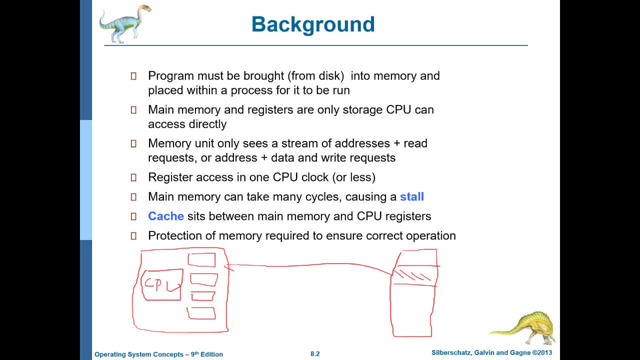 come from the ram into the registers, to any register, okay, and it will be executed in the register. so cpu will actually directly access the instruction from the register and, as i explained, if it is going to get the data from the main memory, it will take some time, resulting in a stall. 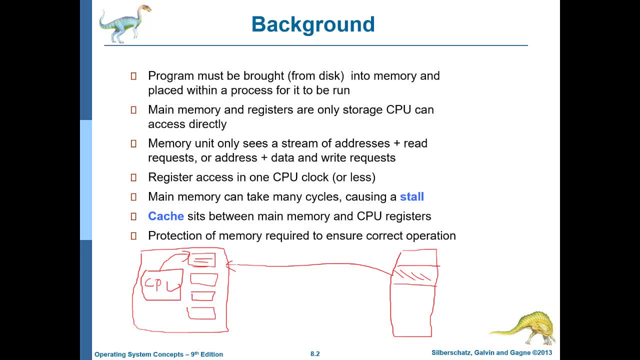 to actually reduce that. what we have is that between the cpu and the memory, we have something, what what we call as cache. okay, so cache memory. why is cache memory useful? because the cache, sorry. so we have this cache. i cannot write it here somehow. cache c, a, c, h, e. okay, now this cache memory, it will. 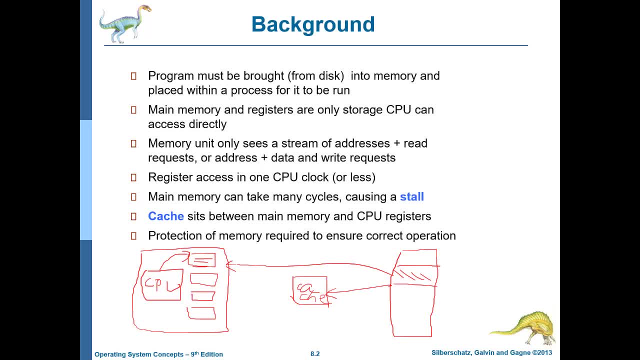 get the data from the ram, okay. and then because it will get many instructions at the same time, so one by one, all these instructions will come into the cpu. now this access from cpu to the cache is passed, compared to the access from cpu to memory, which is quite slow. so that's why cache is useful now. 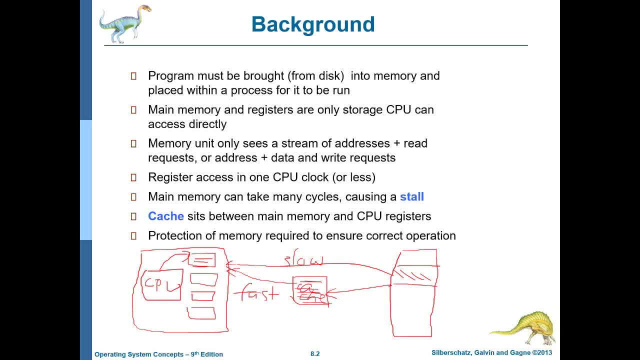 because in the ram there can be many programs at the same time, so this one is one program or process. then we can have another process and we can have yet another process in the ram. okay, so these different processes, they belong to different programs, and we do not want that. any process can. 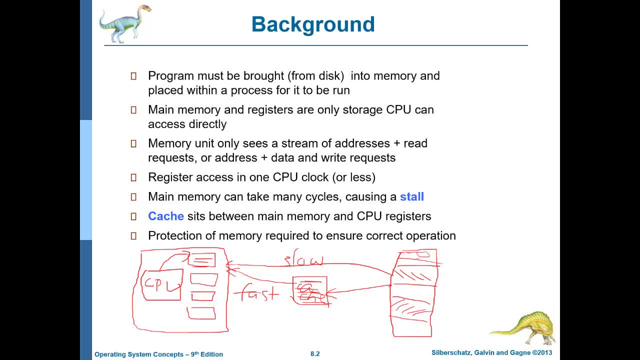 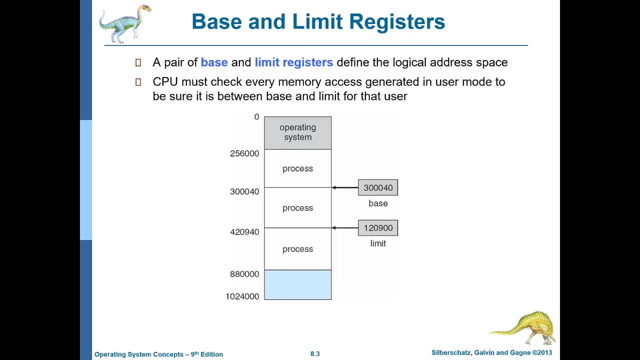 access the address of another process because this can lead to security problem. we don't want this security problem to happen, so we want memory protection. we want that a process can or should only access its own addresses and not any address outside its area. so, for example, here we see that in this ram. 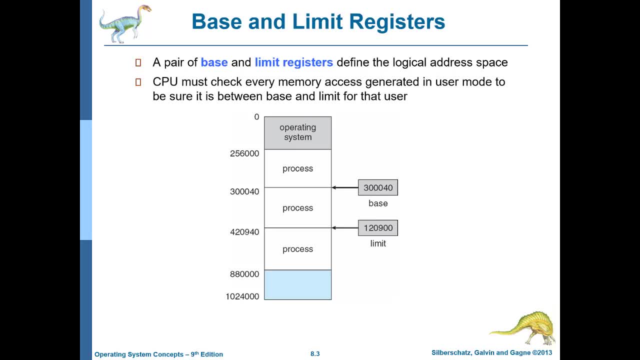 we have three processes. okay, each process has its own address area, okay, which is denoted by what you can see, these address numbers. so, for example, the operating system is in the address area which starts from zero to two, five, six, triple, zero. in this memory area you have the operating system. 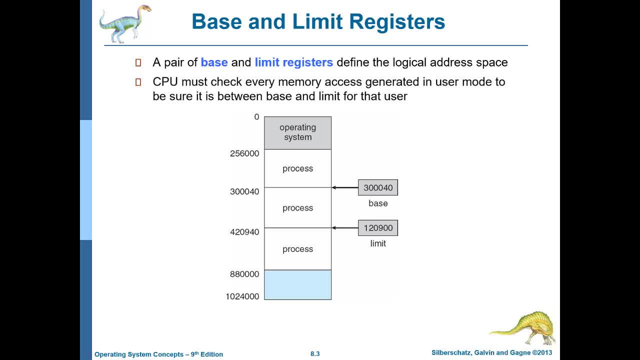 then you have another process. let's call it process a, for example. so this process a, it has the address from two, five, six, triple zero to three, zero, zero, four, zero. this total area, okay, is actually the address of this process, okay, and this process is here. now, what we have. 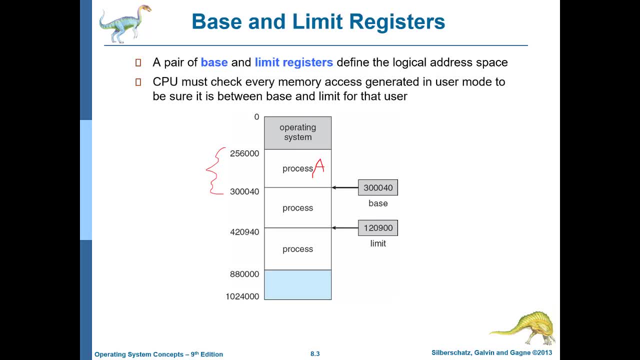 is that the cpu must be executing instructions of process a which are only within this range, which are only from two, five, six, triple, zero to three, zero, zero, zero, four, zero, which is the operating. Similarly, for process B, the CPU must execute only those instructions which are in the range. 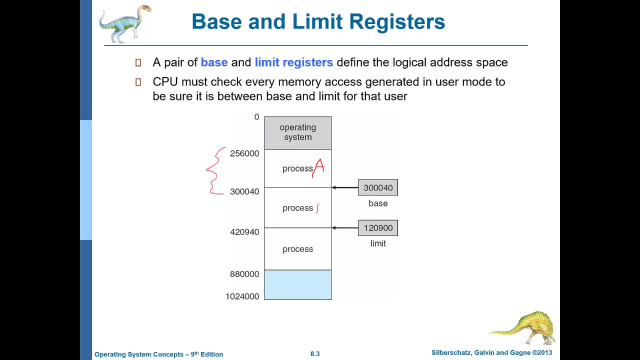 of this, 30040 until 1209000,. this is for process B. So how does the CPU know about them? For this purpose, the CPU has something which is called the base register and the control, the limit register. So the base register and the limit registers, they have the value of those areas within. 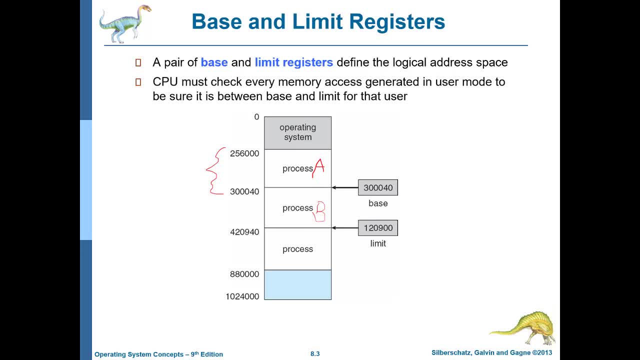 which this process is residing in the line. So here you see that process B is between these limits of base and limit register. Now, whenever the CPU wants to make a reference for process B, it will make sure that it is more than the base and less than the limit. 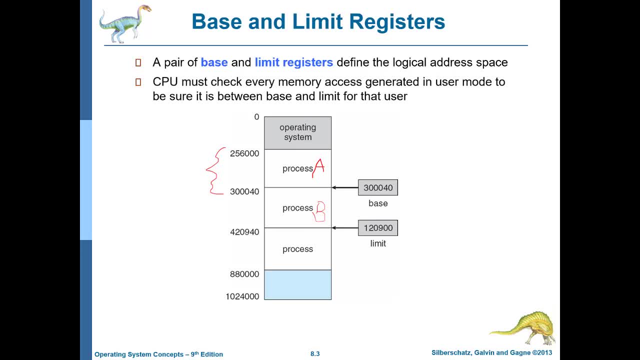 So on the left side of the RAM what you see is actually the memory addresses and on the right side the base and the limit. So this is the memory address. So this is the memory address. These are the registers. So the base address here is same as the address on the left: 300040.. 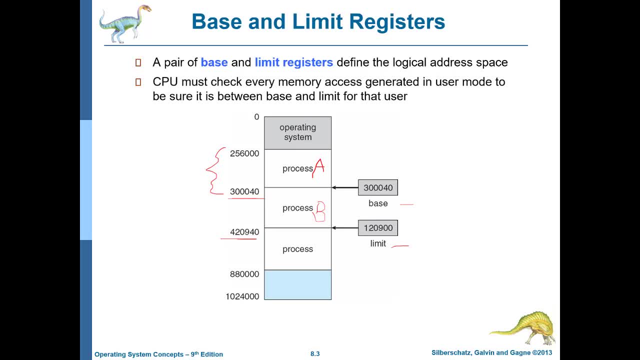 But the limit is different for the address and the limit register. Why is it that? Can anyone tell me? Actually, the reason is, if you add the base number to the base number, the limit register and the limit, so together they will give you the same number, which is 420940, which. 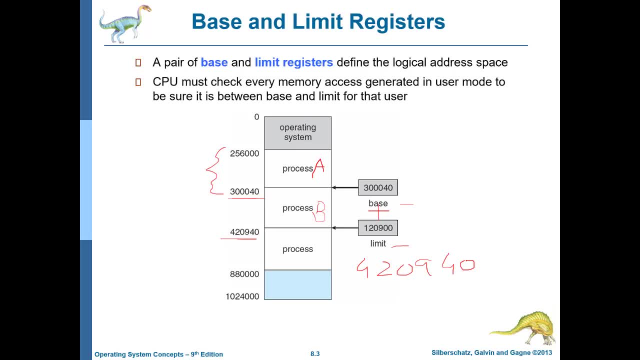 is this number on the left. So it means that this limit actually represents the size of the process in the RAM. So the size of this process is 120900.. Every time the CPU wants to have an instruction from process B, it will be within these addresses. 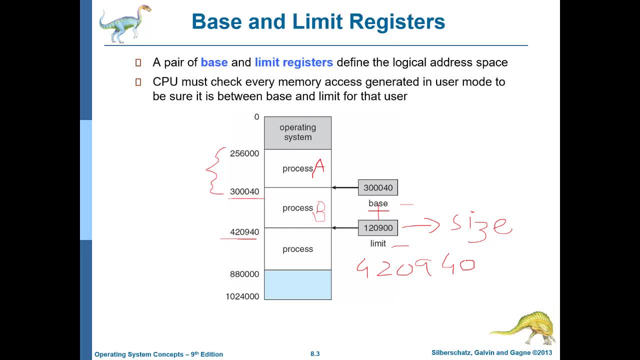 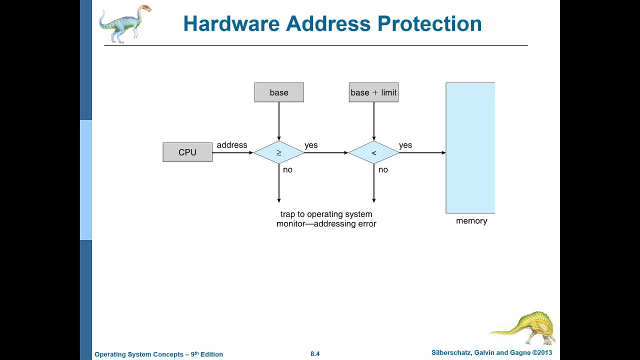 from 3000040 to 120900.. How does a CPU do that? Actually, this is done by hardware address protection unit of the memory and what happens is that: 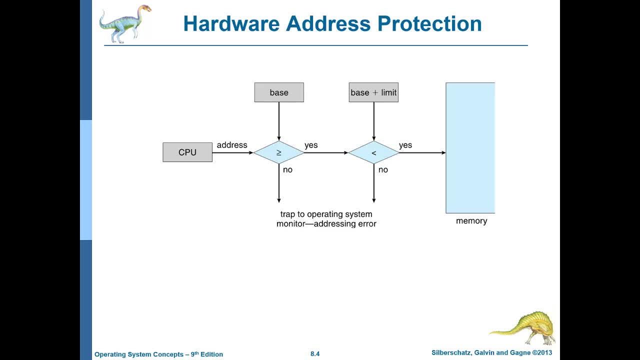 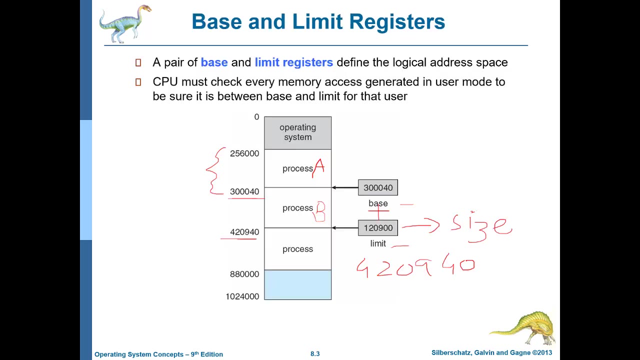 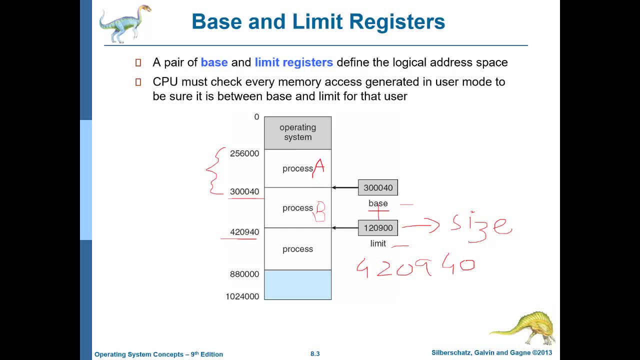 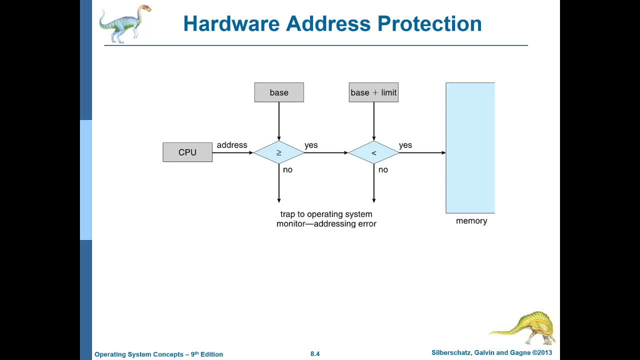 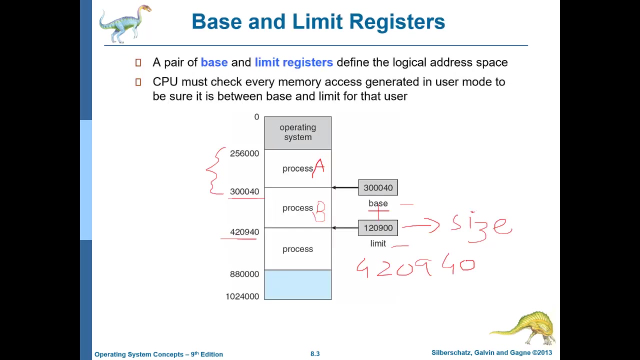 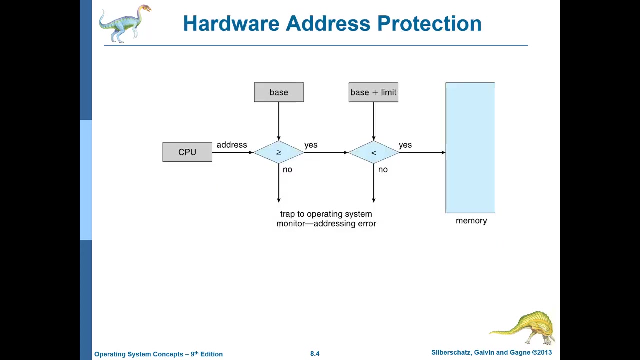 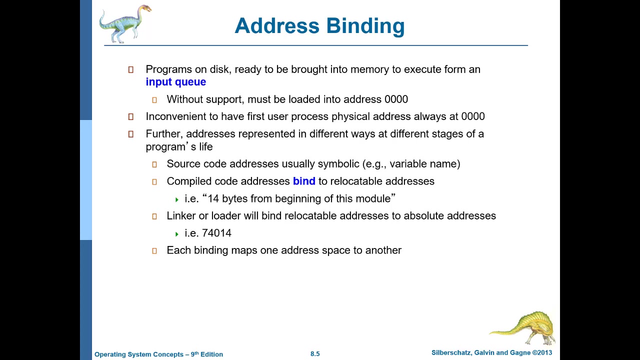 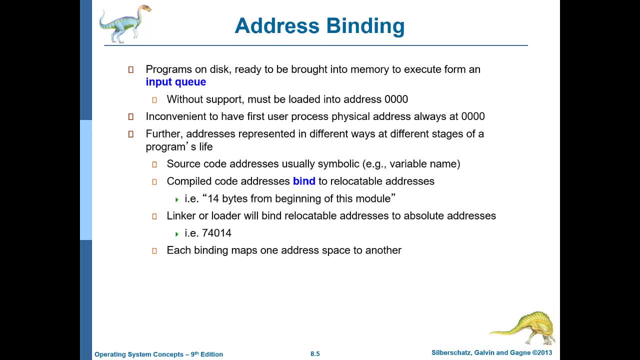 So it will always be stored in a relocatable code. We refer to an address starting from some starting address. For example, the very first address in a program is 0.. 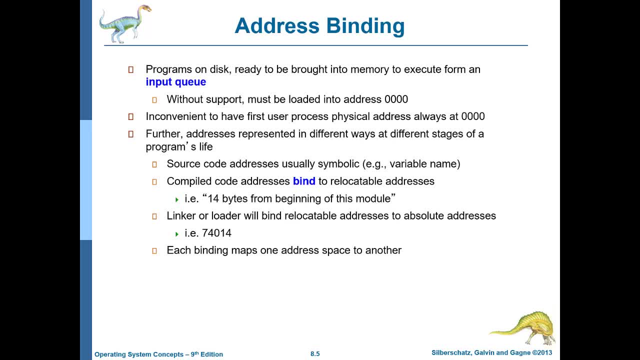 Then in a relocatable code we will say that this instruction is located 14 bytes from beginning, or this instruction is located 100 bytes from the start of the program. This is relocatable. Why is a relocatable address needed? Because when you run the program it is loaded into memory. It does not know where is this in the memory, but it will always refer to the start of the program as the starting address and the next instruction will depend on the starting value of the address. 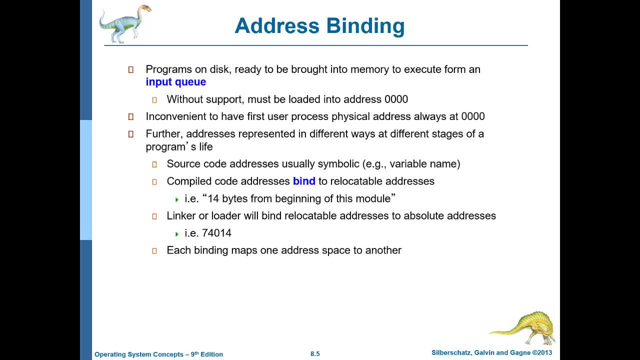 This is the compiled code. Then the linker or the loader. it will bind the relocatable address to absolute addresses. For example, the actual program can be loaded into memory location 7400.. So the relocatable code at 14 bytes will be at the address of 74014.. It is 14 bytes from the starting address which is 74014.. It does not know where is this in the memory. We refer to an address starting from some starting address, which is 74014.. Then the linker, or the loader. it will bind the relocatable address to absolute addresses. For example, the actual program can be loaded into memory location 7400.. 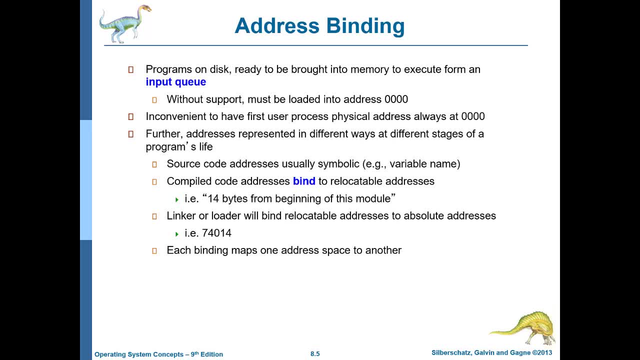 This is the compiled code. Then the linker or the loader. it will bind the relocatable address to absolute addresses, which is 74014.. So the relocatable address can be loaded into memory location 7400.. That is what I meant by gekommen. 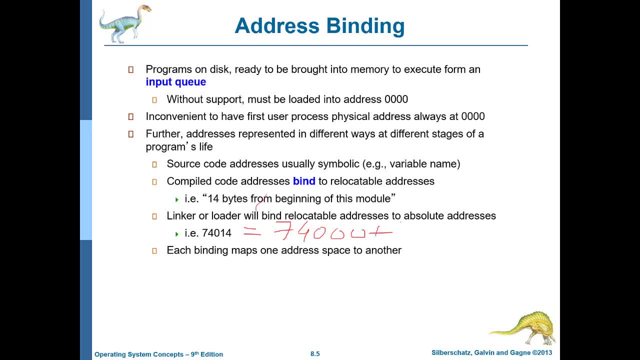 That is why, when you open the linker or the loader, it will see the escalation from 74014 to German. So basically, you cannot remove the linked address without beingicy of this Hindi East, English and Englishian language from start to end. What you should be aware of is that each of these loss is Löws. 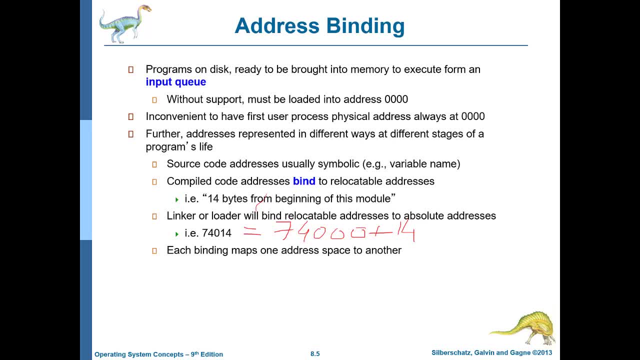 This happened only after when I created께 tarWith numa, Evergreen or mari, and this conversion of address from, let's say, relocatable to absolute addresses. this is known as address binding. so we have different types of binding. one binding is from variable name to. 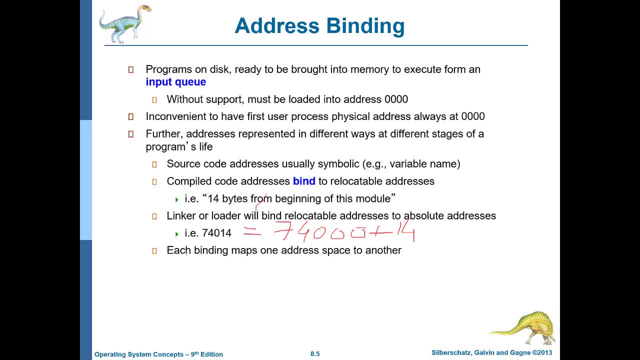 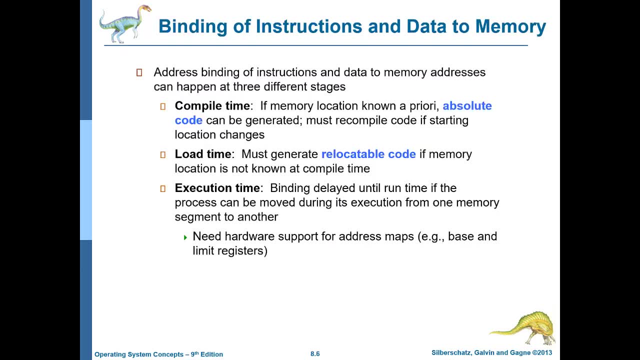 relocatable address and the other one is from relocatable addresses to the physical addresses, and this binding is both for instructions and data. in a program you can have instructions, for example print or see in, etc. these are the program codes- or it can be about data, which is the variance. 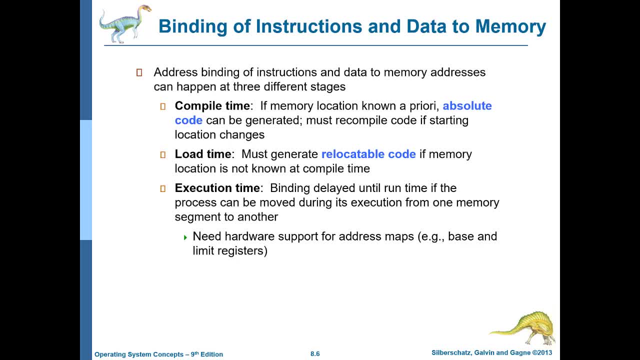 of the program. now this binding of instructions and data can happen, and three different times. The first it can happen is at the compile time, which means that if memory location is known in advance, then you can generate absolute code. So let's say, we know that a program 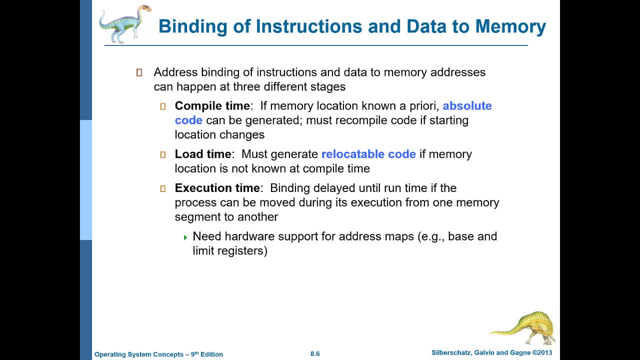 will be executed at address number 100. It will be loaded, started from address 100. Then we can have an absolute code in which we write: let's start the program from address 100.. But actually it does not work like this, because you are not sure at the compile time that what will. 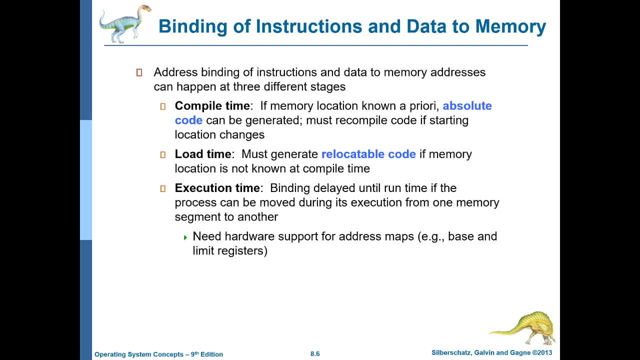 be your address of execution. So the next thing is to have actually these addresses bound at the load time. This binding takes place at the load time when you load the program into the RAM, And in that case we must have the relocatable code, which means that we don't know. 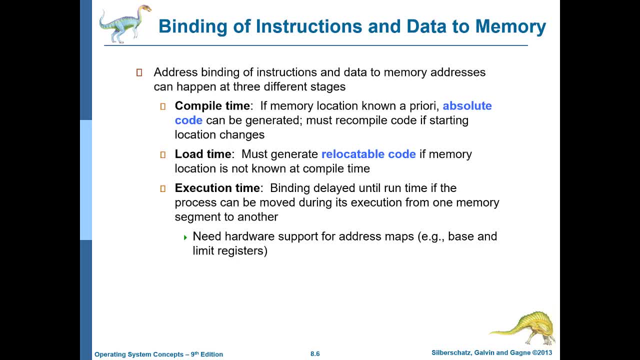 about the starting address in which this program will be loaded, But we will generate a code with respect to any starting position, So this program can be anywhere and we will know that wherever this program is, I will refer to an instruction with respect to the starting position of the program. Then the third thing is about execution. 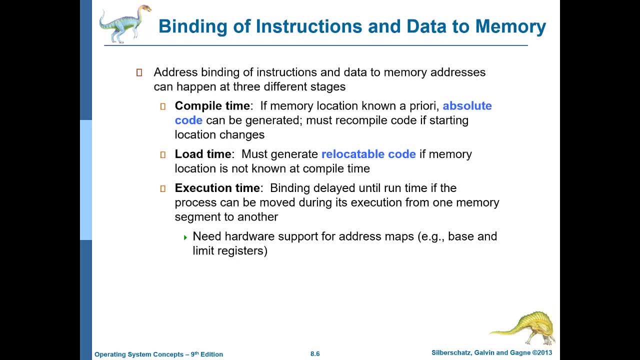 time, Which means that the binding is delayed until the run time. if the process can be moved during execution from one memory segment to another memory segment- And this is what is happening in the modern operating system- That your program can move in different locations in memory when it is executed, And for this to happen- the execution time binding- we need support. 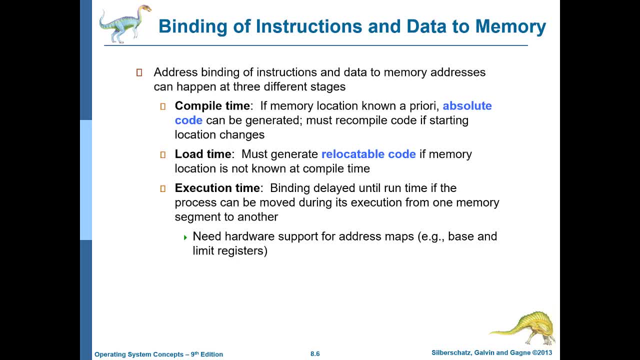 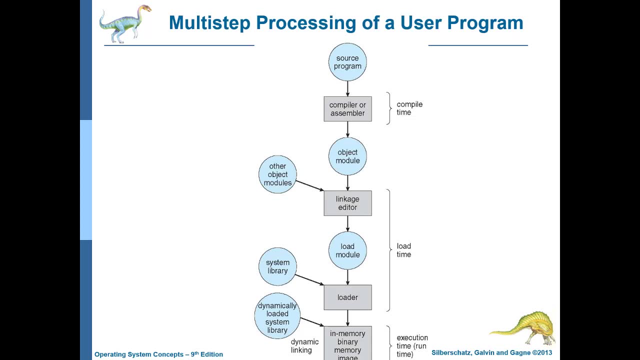 from hardware for mapping of these addresses, And this is done in the example of base and limit registers that I explained before. So this diagram represents the whole schemes that if we have a source program and we are considering compile time binding, then this address will bind at the level of compiler or assembler And this will result in an object module which will 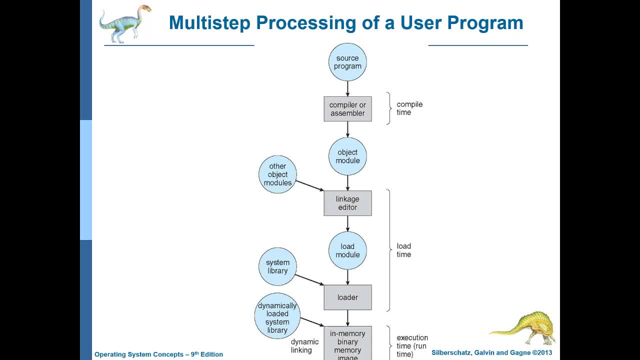 have fixed binding. Similarly in the linkage editor it links actually your object modules to other object modules, Which means that within your program you write your own code. that will be your object module, But your code will include some other object modules. So in this example we will: 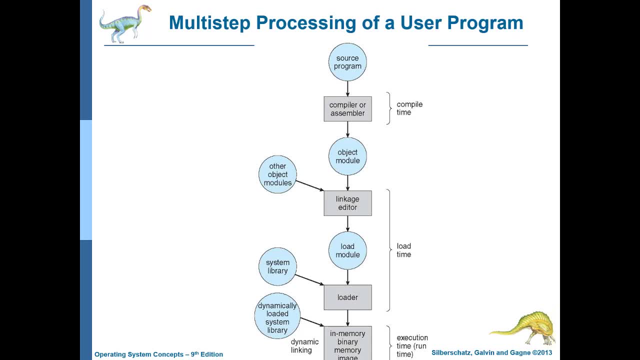 use some other object modules from the programming language, This linkage is done and you load the module. So all this processing is done at the load time. Now the loader is an entity which will actually combine the load module with the system library by the operating system. 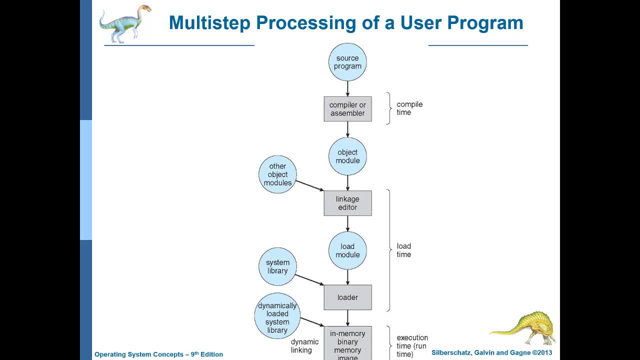 And in the memory you will have the image of the program. But during the runtime or the execution time this program image it will need access to dynamic linking to dynamically loaded system library. An example is a DLL file. Now a DLL file is present in the operating system and when a program needs services, they 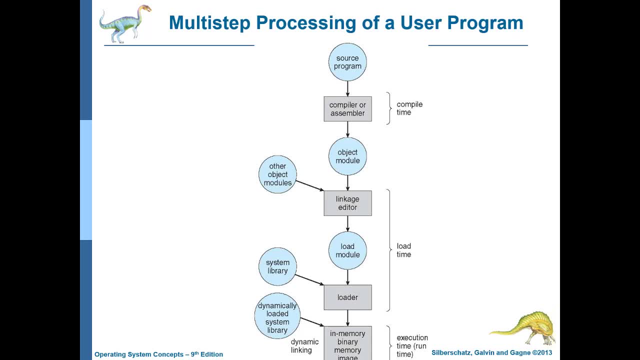 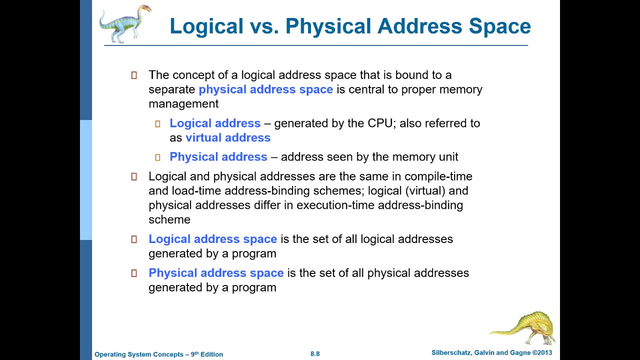 load from the dll file, and these dll file are normally available at different locations in the operating system and used by the programs. so now we need to distinguish between two types of address spaces. one is known as the logical address space, the other one is known as the physical. 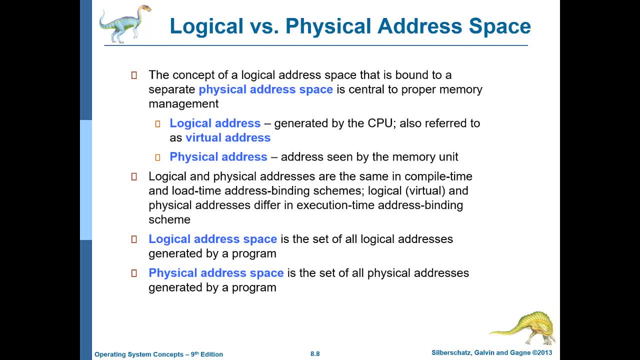 address space. so a logical address space is different for each process, while a physical address space is same for the whole system. why is it different for each process? because a logical address space means that when you load a process into ram, so for that process because it only knows its own addresses. 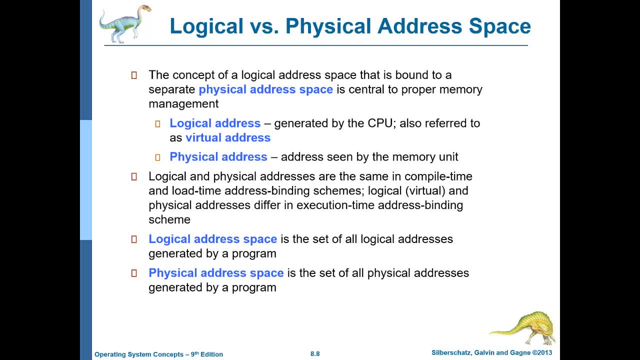 for it the starting address is always zero and the ending address is the limit of that process. that is the logical address space and the other one is physical address space, which is actually the address space seen by the memory unit which consists of the ram in the system. so what cpu does is actually generates the logical address space. 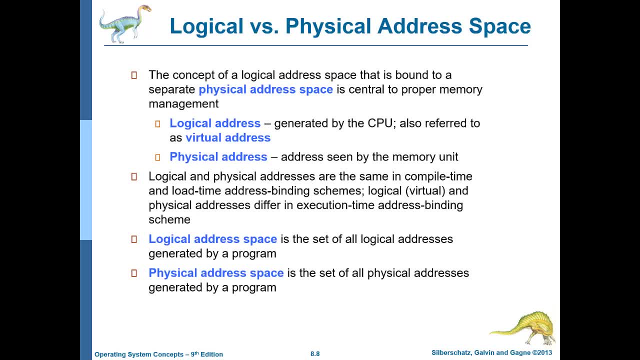 inside each process. so it will say that execute instruction number five in this process or execute instruction number, for example, 50 in this process. so it will send the address of the instruction in this process to the memory unit and this will be known as the virtual address or the logical address. now the memory unit will take this. 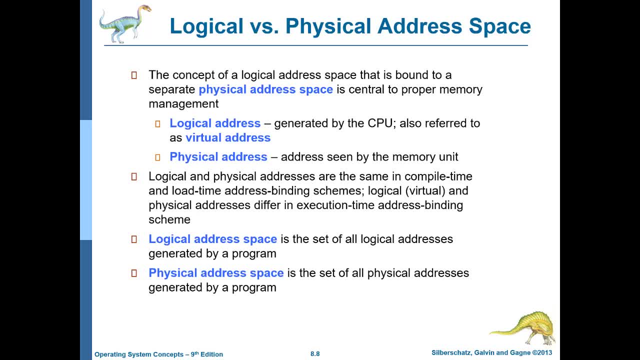 virtual or logical address and it will convert it into a physical address which will be in the ram. then the data or the instruction at that physical address will be fetched from the ram and loaded into the memory. so logical and physical addresses are the same in compile time or load time. address space. 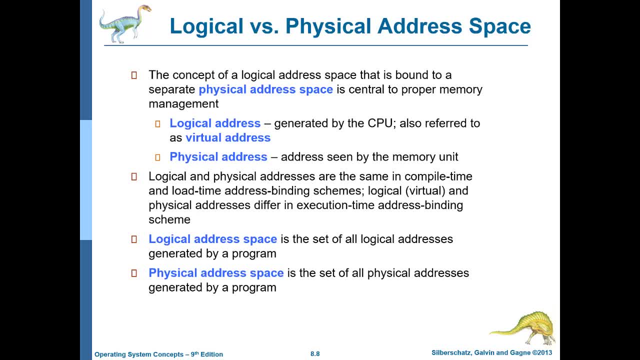 address binding schemes, But in the execution time and address binding scheme they are different. Logical address is different and physical address is different. So the logical address space is actually set of all logical addresses generated by the program, which is limited by its size, starting from address 0. And the physical address space is the set of all physical. 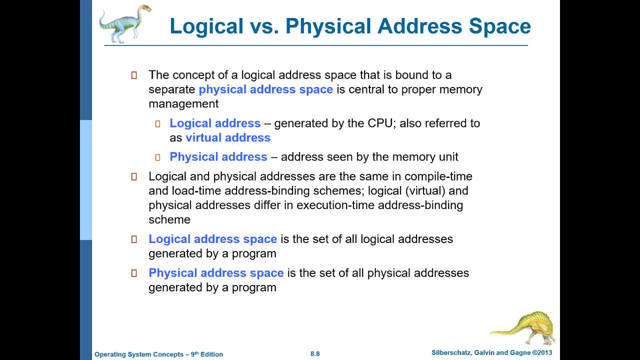 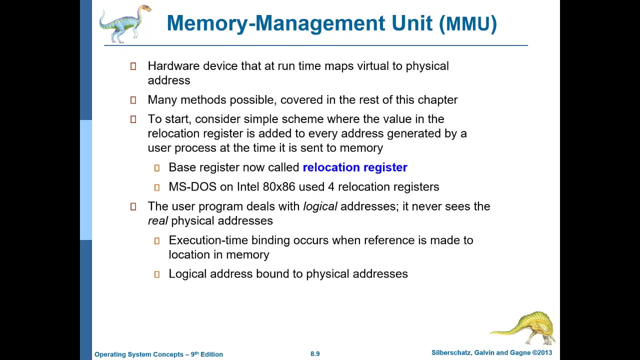 addresses generated by the program. If we don't consider virtual memory, then this is the random access memory, the size of the random access memory in which this program can be placed anywhere in the RAM. Now we should understand the role of the Memory Management Unit. What is the Memory Management Unit? It is a hardware device that maps the virtual 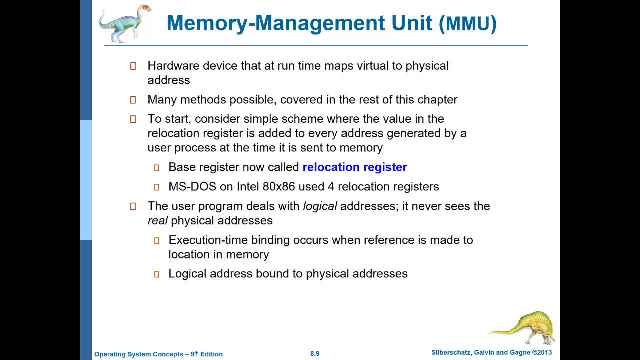 memory address to physical memory address at runtime and there are different methods to map this virtual address into a physical address and we will see those schemes in the rest of this chapter. so, for example, we consider a simple scheme where we have the value in the relocation register which is the 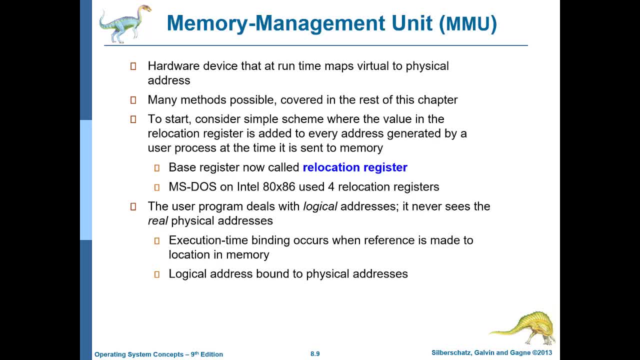 starting address of a process and then we add the value of the relocation address to every address generated by the CPU. because of CPU we tell greater logical address and to get the physical address we will add the logical address with the relocation address value and then the final value will be some. 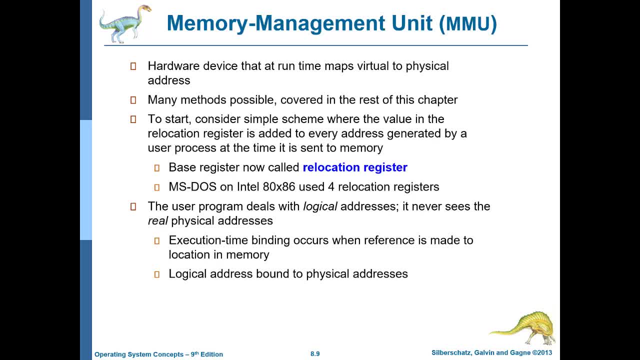 physical address in the main memory. now this is known as the relocation address address. we don't call it a base register now. we call it as the relocation register because it will give us the addresses according to the position of the process in memory. so if we consider anastas operating system then it would use four relocation addresses. 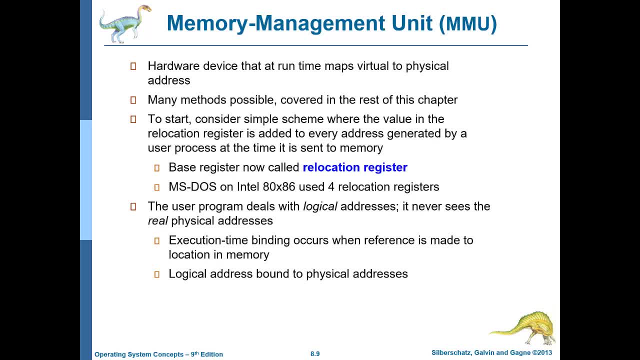 now modern operating systems. they use different number of relocation registers. so for a user program it only knows about its own addresses, and these are the virtual or logical addresses which always start from the first instruction which is at position 0, and it goes until the size of the program. for a process there is nothing more than. 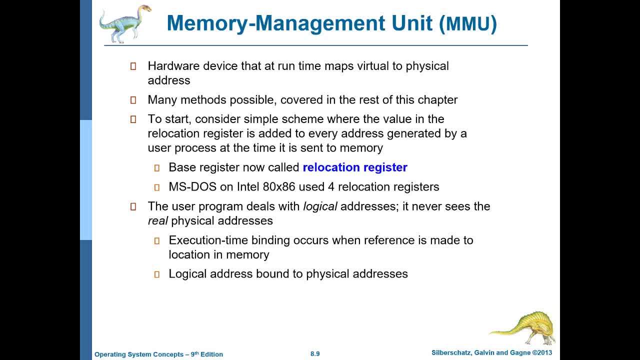 its own addresses. it does not know anything about other processes in the ram or the size of the ram etc. it only has its own world in terms of its own addresses in the main memory. so in execution time binding when the cpu makes a reference to a memory location. 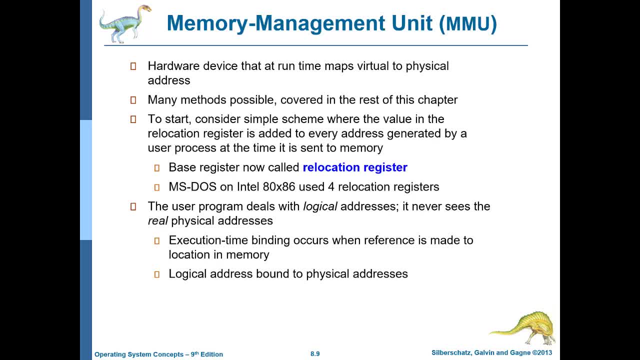 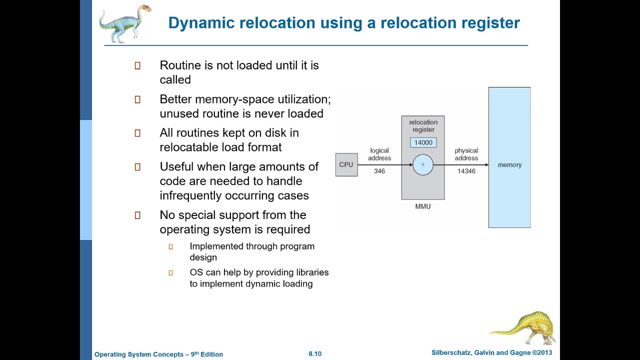 then this binding occurs, which means that at that time a translation is made from the logical address to physical address. in this way, the logical address is: they are bound to physical addresses. now here we see the example of dynamic relocation using a relocation address. so the relocation address: it contains the starting address or process in the relocation register. 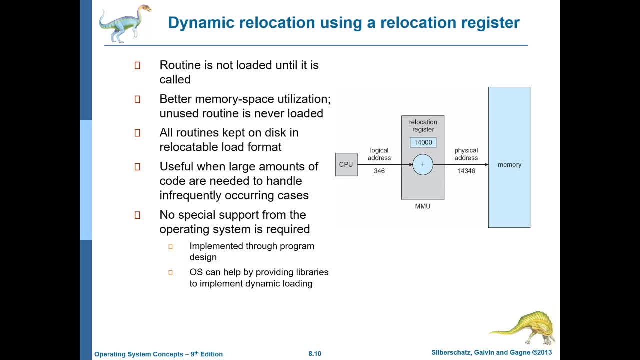 so within the logical address of a process, a process may be executing the instruction number 346. so the cpu sends the logical address of 346 to the memory management unit. the memory management unit will take the logical address and will add it to the relocation address to give us the physical address in memory where we can get this from. 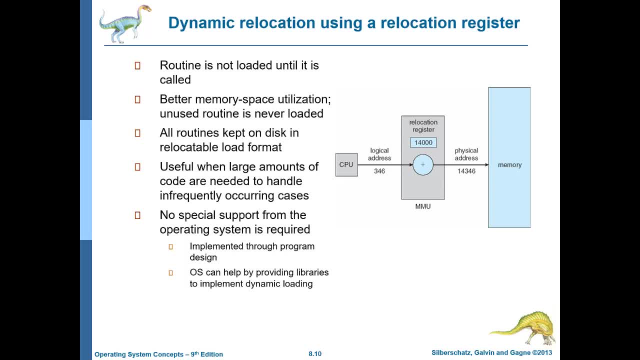 the memory management unit. so all this mapping from logical address to physical address is done by the memory management unit, which is hardware and it is. it does not require any special support from the operating system. the operating system can help in the operation of the memory management unit. 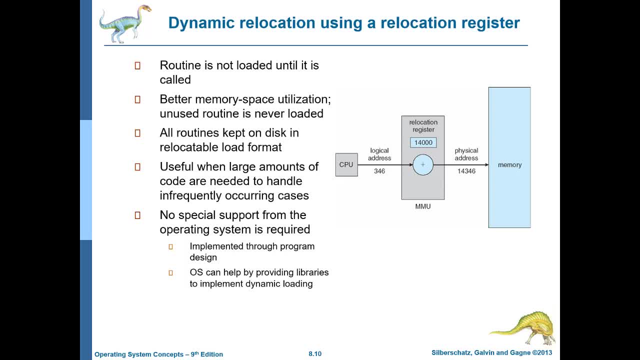 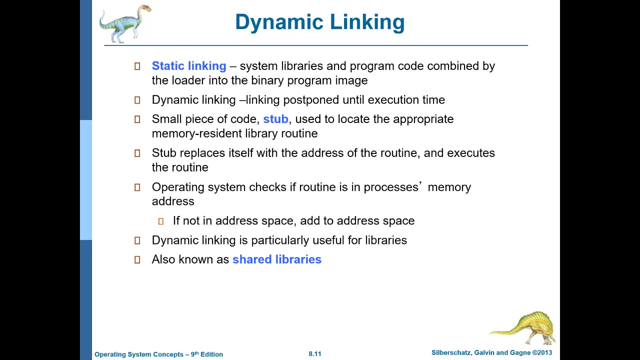 the dynamic loading of the program into different areas of the memory. once a process is in memory, then the job of the memory unit is to translate the logical address of that process into the physical address. now we have the concept of dynamic linking and static linking. what is static linking? static linking means that the system libraries and the program code 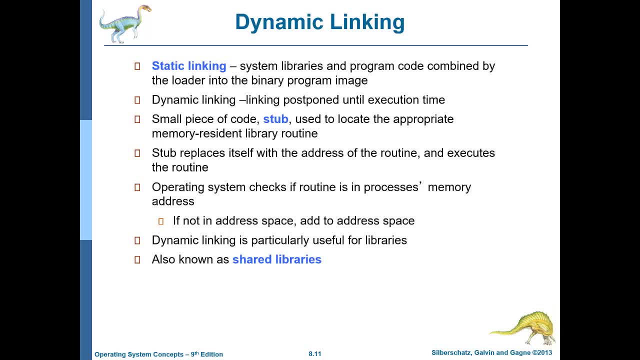 which is written by user. they are combined by the loader into the binary program image, so the system libraries become part of the binary program. when you load the program, that system will be loaded into the binary program. that's why you have static linking the program. the system libraries are loaded inside the program. There is no. 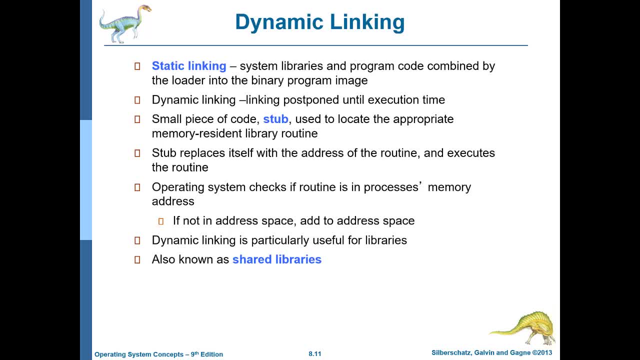 need to call additional libraries from the program because they are inside the program. This is the concept of static linking. In the dynamic linking the system, libraries are not linked with the main program and this linking is done at the time of execution. Now there is a small piece of code which is called 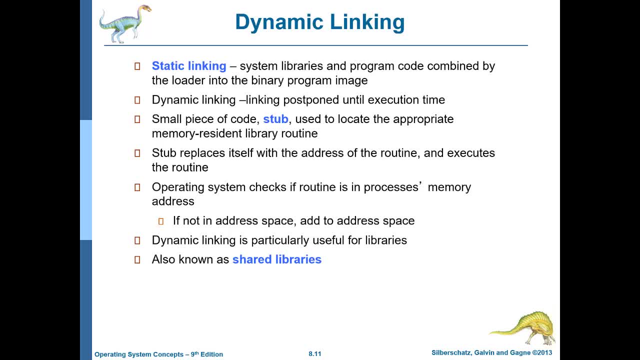 stub and this is used to locate the appropriate memory resident library routine. Its job is to find where can it find this system libraries. It contains the information about system libraries or it can communicate with the operating system to get to the libraries Now when you run the program. so initially the stub is there inside the 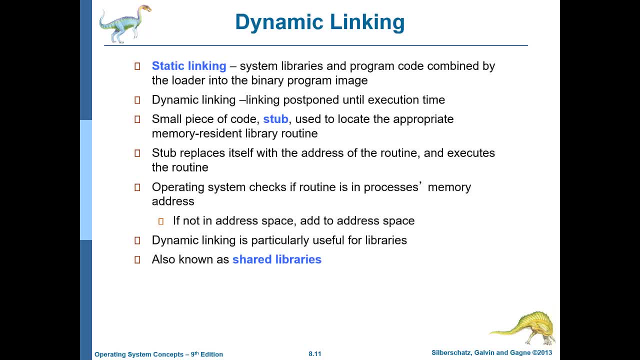 main memory, but once there is a need to execute the system libraries. so the stub will replace itself with the address of the routines in the system library. A routine is actually small part of a program. Now the operating system will check if the routine is which is needed by the process. It is there in the processes memory address. 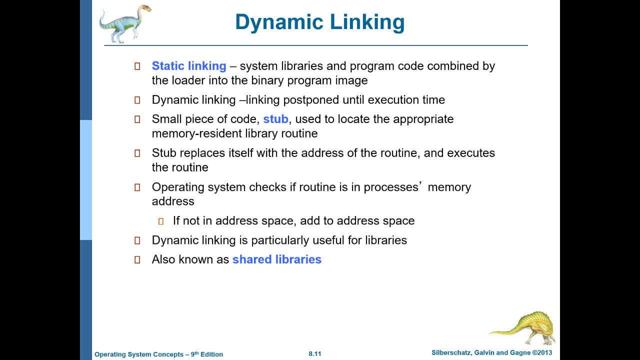 space already, then it will run the routine from there. If it is not in the address space, then it will add the routine to the address space. So the dynamic linking is very useful for libraries. It is used quite significantly in the Windows operating system in the form of dynamic linking. 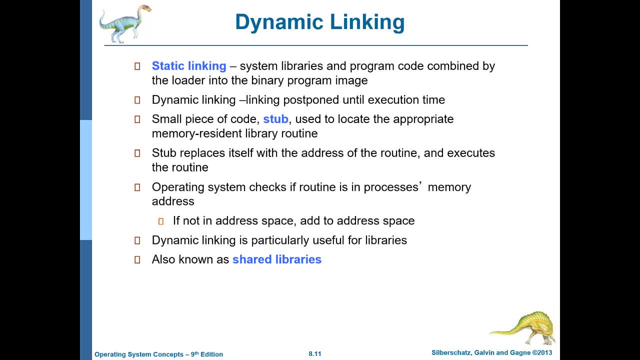 We can see the process file or the process and the dynamic link libraries file or the DLL file. These DLL files are also known as the shared libraries because they are shared between different processes, So they are present in the operating system. when we load any program and they need these libraries, a reference is made to 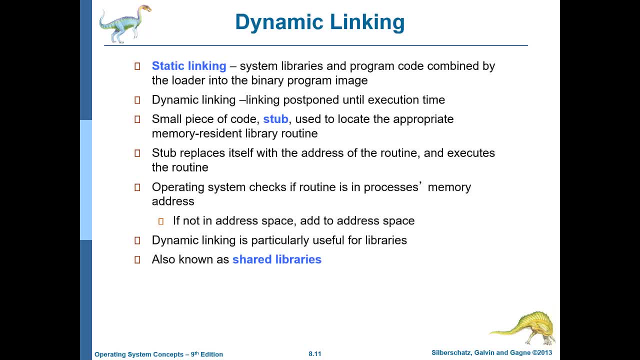 the library by the program and the library is included in the process. So if program for use by the, this program, so we stop here and then next time we start with swapping. if you have any question, you can ask me.